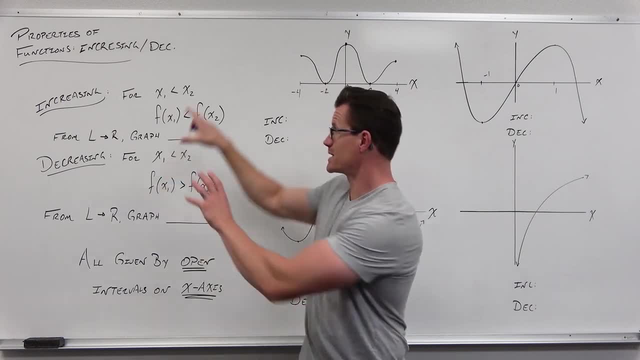 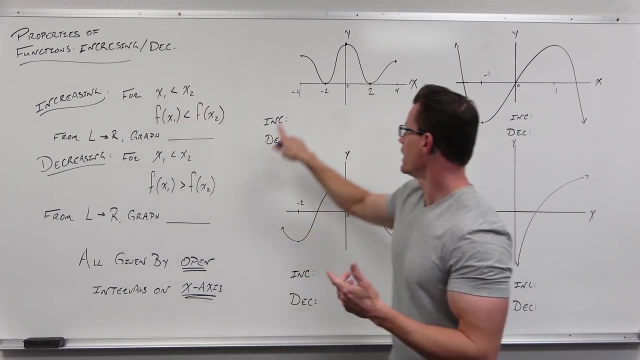 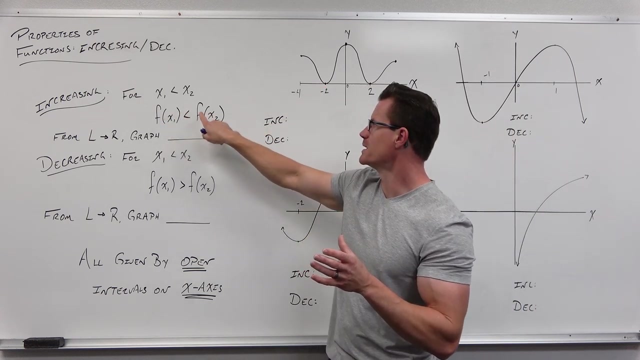 will be larger as you move to the right. That's what this says in English. It says as you look from left to right. so an x value and one bigger than it as you look from left to right. what's your function doing? If a function's increasing, then the output will be getting larger as you. 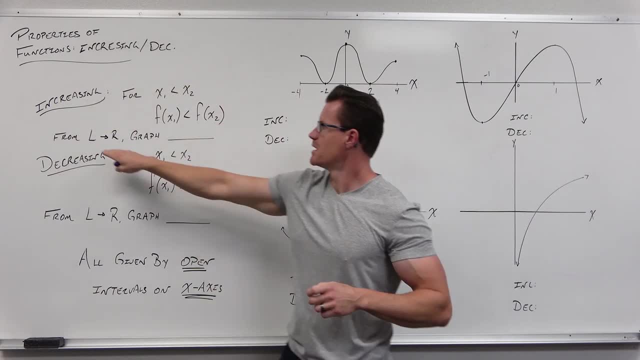 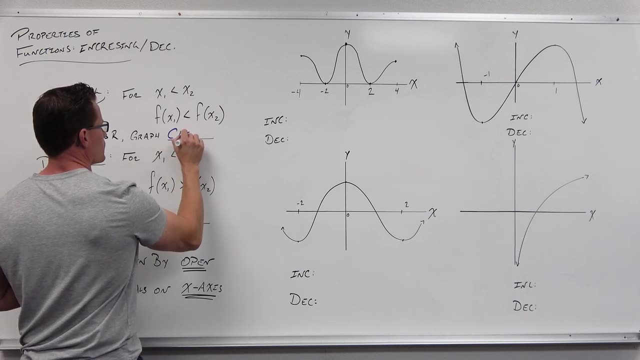 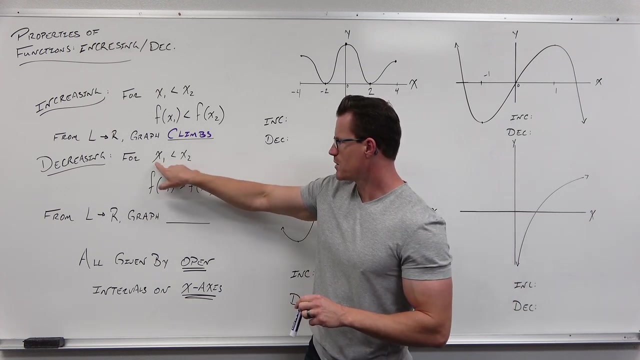 move from left to right. So in English, what this says is: from left to right, the growth graph climbs. That's what increasing means For decreasing. the opposite happens. This says: hey, look at your x values. If you have an x value that is getting larger as you move from left to right. 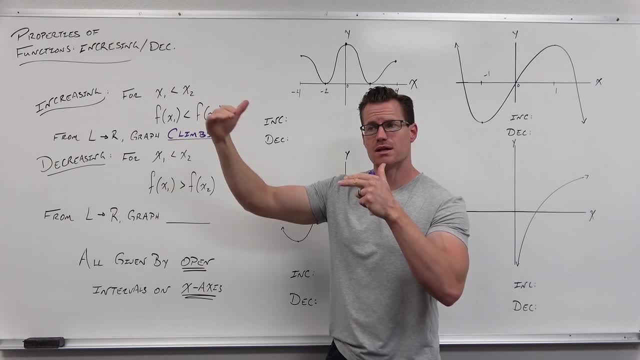 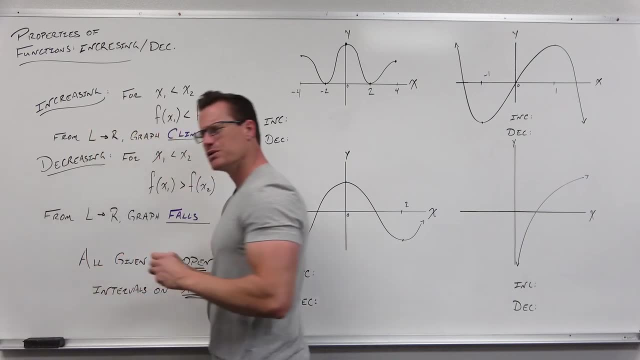 then your output will be getting smaller and that would create this graph that is falling as we move from left to right. A couple notes to really keep in mind. All of this is given by a function. So if I take a look at an x value and one to the right of it, all of this is given by. 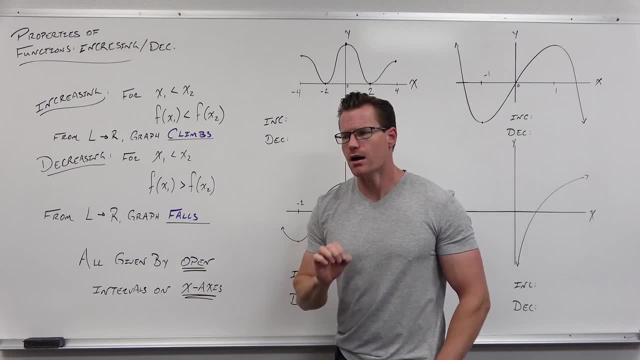 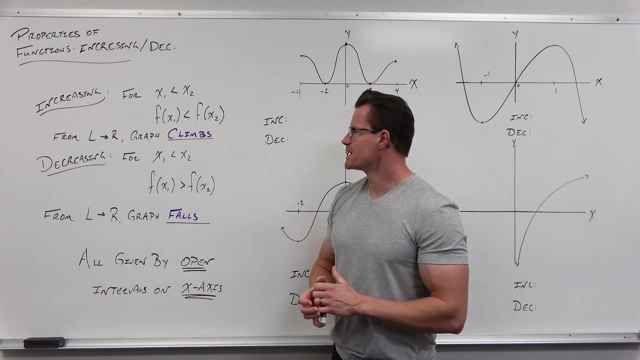 an open interval. You will never, ever use brackets or equal signs with increasing and decreasing, And the reason why is because, if we're increasing, it has a connotation that as we're moving from left to right, the graph continues to climb and climb, and climb and climb. 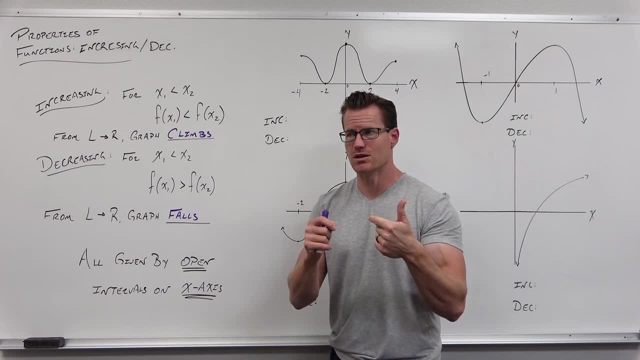 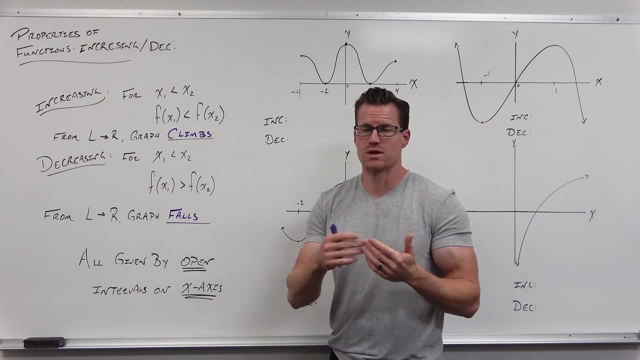 That means that the next value has to be bigger than the previous one and you can't stop or create this closed interval and have an increasing idea. It could have increased until that point, but it can't be increased until that point. So if I take a look at an x value and one to the right, 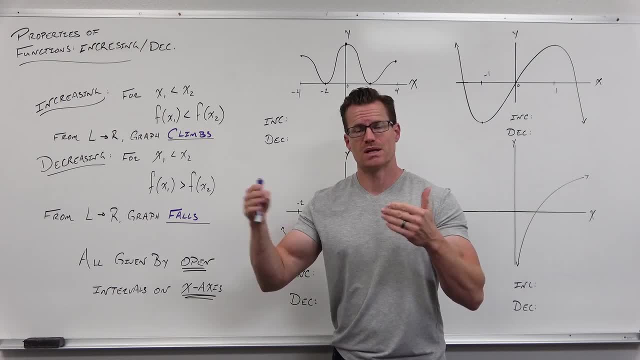 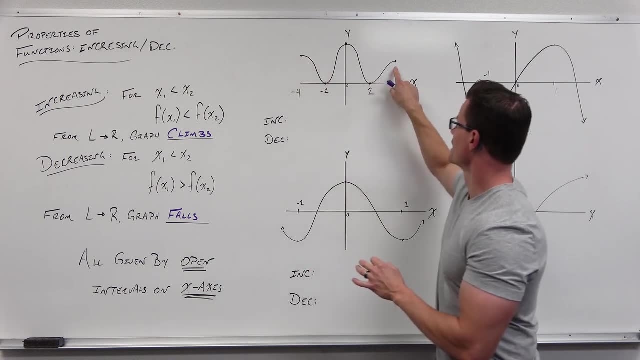 it's increasing because the next value would not be there And so we can't check to see, well, what's the next value? Pass an endpoint. So if we have an endpoint, you can't say it's increasing at that endpoint because there's no next value to test whether to see if the output 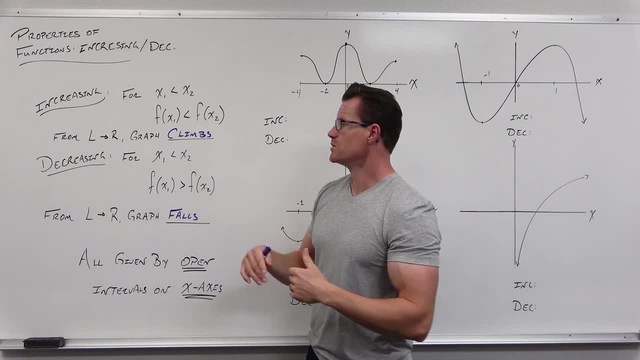 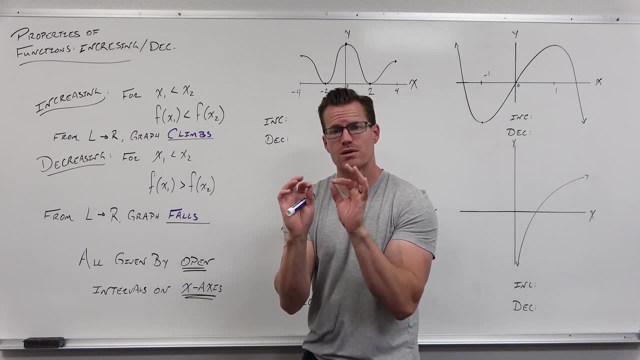 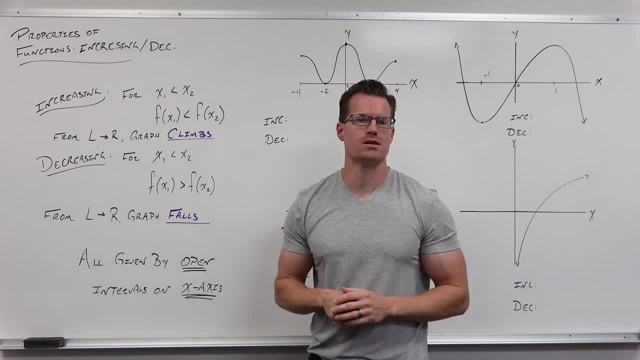 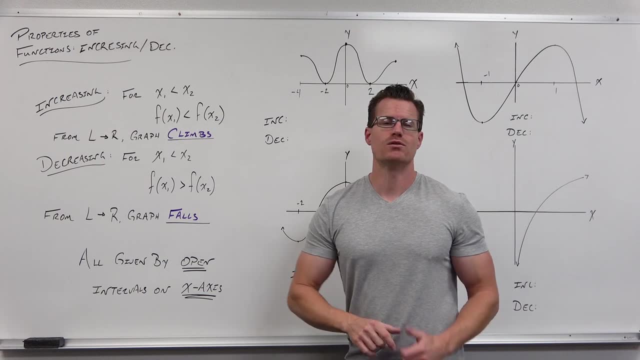 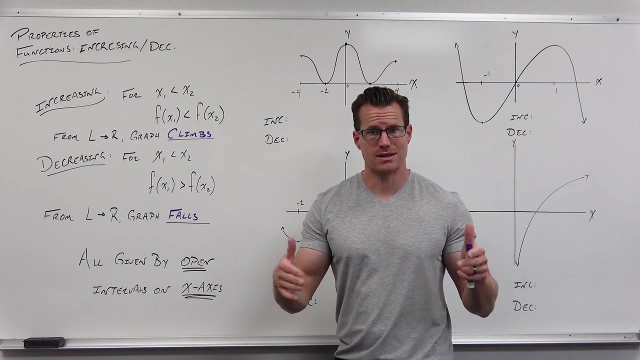 or smaller and smaller. You can't do that if we start closing things off. So all of our intervals are always open for increasing and decreasing and they're always given by the x-axis. Do you remember me telling you that how a lot of things in graphs are determined by the x-axis? Really only a range. 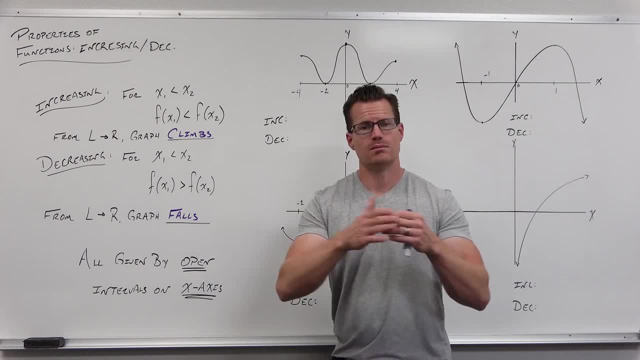 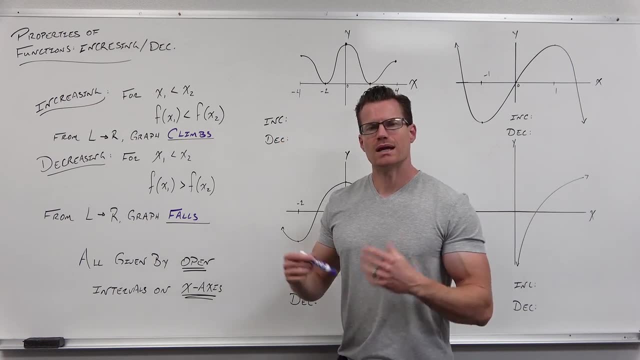 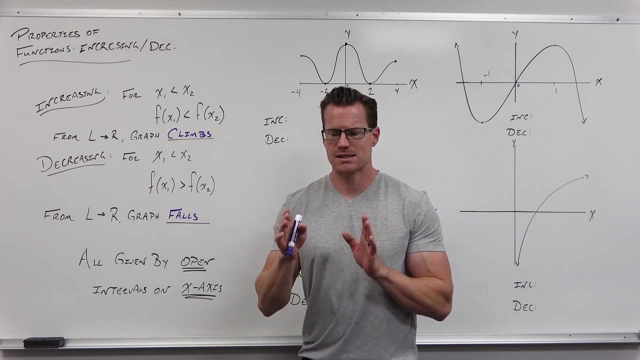 a couple of other things determined by the y-axis idea, but like domain x-axis idea, x-axis idea Where we're above or below the x-axis x-axis idea. So what- increasing and decreasing really ask? in English it is this: Increasing says: tell me the part of the x-axis where, when? 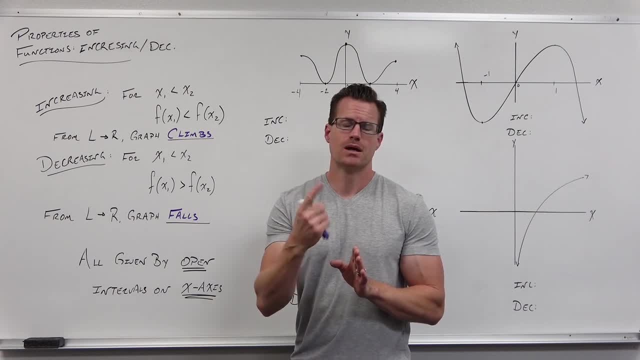 you look from left to right, your graph is climbing. Decreasing says. tell me the part of the x-axis where, if you look from left to right, your graph is falling. That is what increasing and decreasing mean, as simple as I can make it. So we're going to look at some. 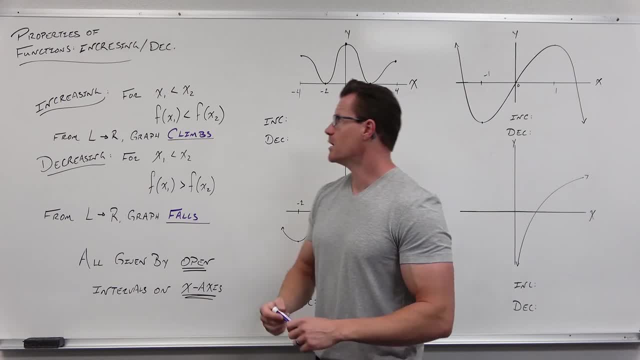 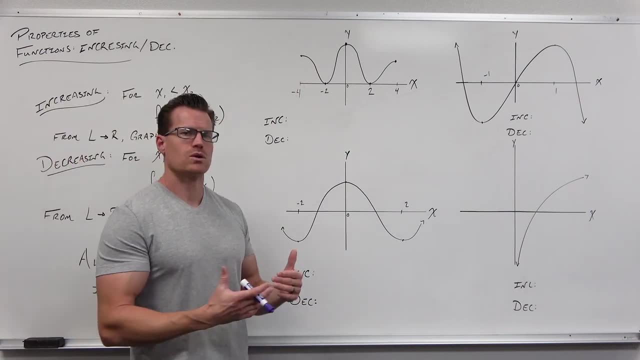 intervals. I'm going to use only interval notation today. You can translate this to any notation, no problem. But let's take a look at this first graph. We want to look for increasing first and then decreasing later. You can do them backwards, it doesn't really matter, But let's 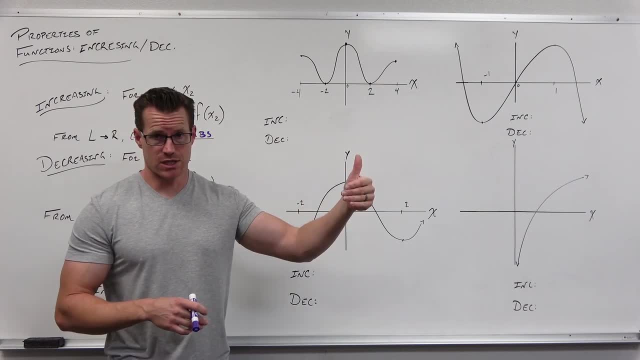 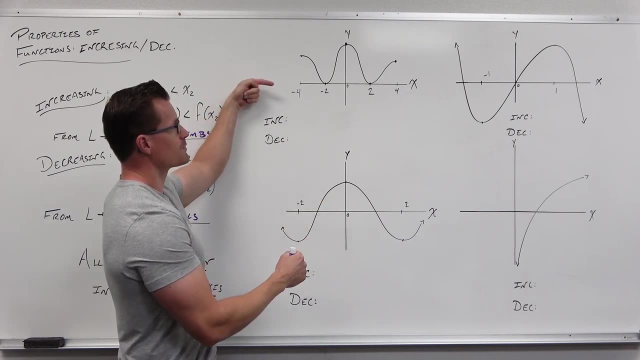 take a look at it. When we say I'm looking for the intervals of increasing, what we're looking for is the interval, the part of the x-axis where, when I read it from left to right, that's what this means left to right. When I read from left to right, my graph is climbing. 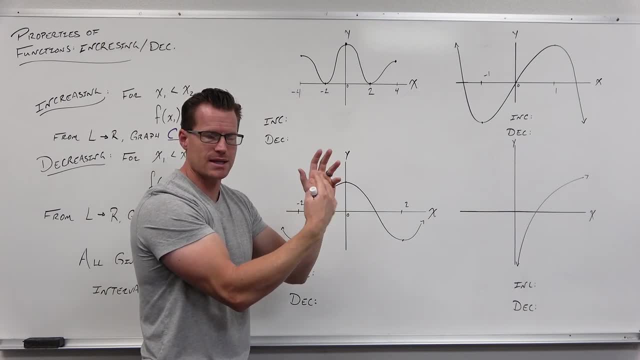 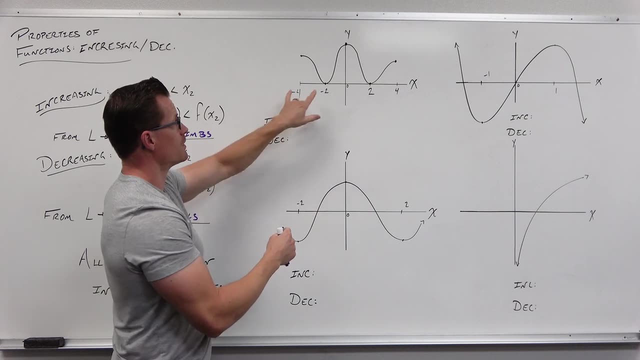 So not right to left, and my graph is climbing. That's not what we're talking about. But it's not what we're talking about. But as I read it from left to right, my graph is climbing. So is the graph climbing on this interval? No, no, no, The graph is falling. As I read from left to 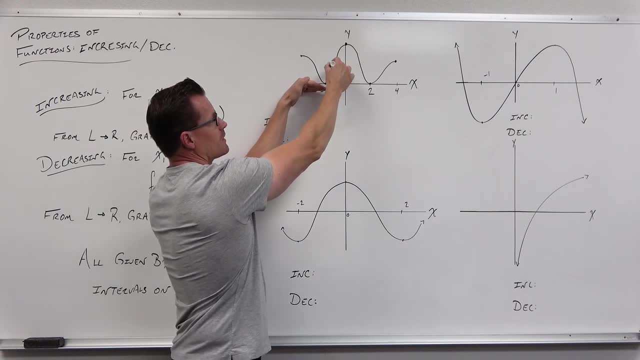 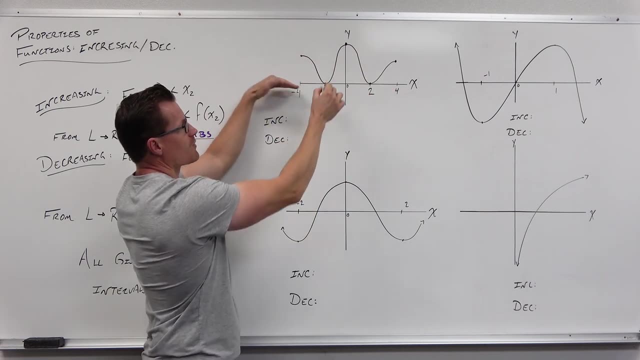 right, this graph is falling, Then I get to here, then it climbs. Then I get to here and then it falls. Then I get to here and then it climbs. Notice, my right hand was tracing the graph but my left hand was looking at my interval on my x-axis. The left hand here is what's. 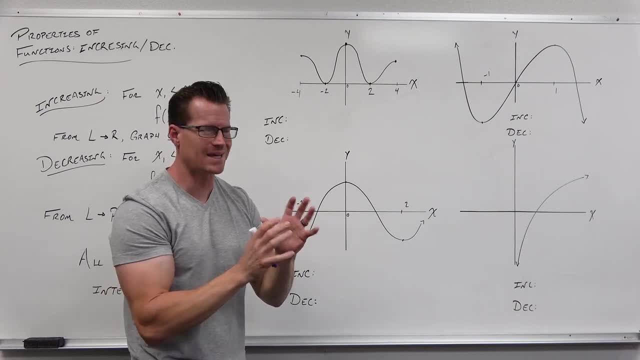 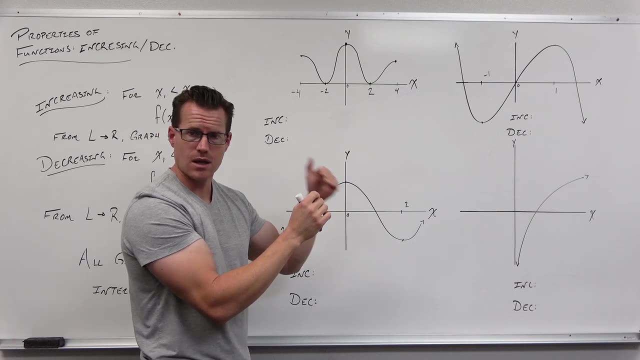 determining your intervals of increasing and decreasing. So again, the x-axis is the section of the x-axis where, as you read it from left to right, my graph is climbing. That's what increasing means. So I'm looking at this, going all right here. 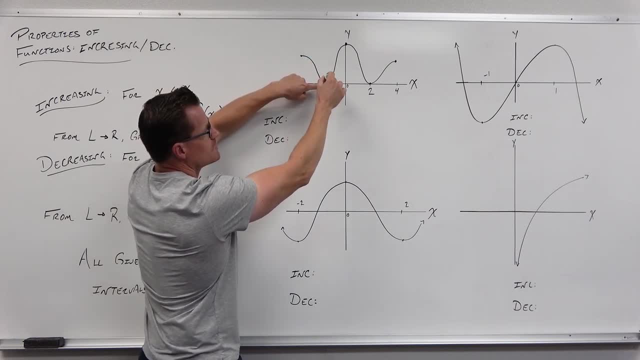 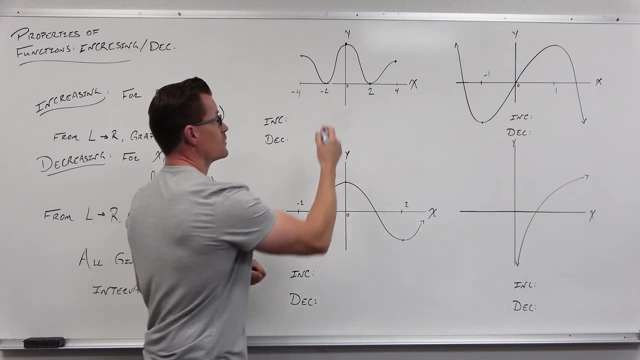 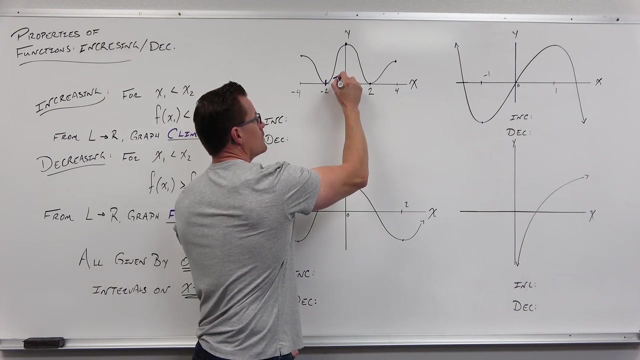 to here. my graph is falling. Oh, right here, right here, at negative 2.. It starts to increase until I get to 0.. So one interval of increasing would be on the x-axis, from negative 2 to 0.. This is increasing. I'm just going to put an i there. 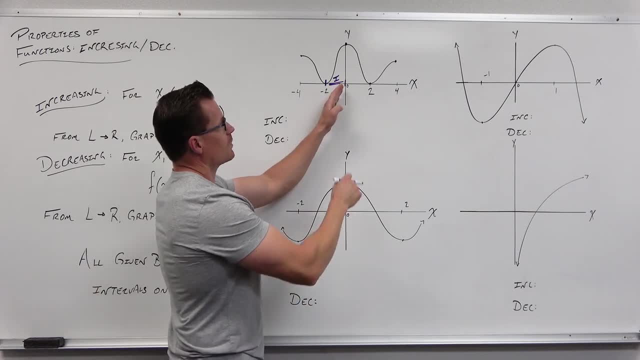 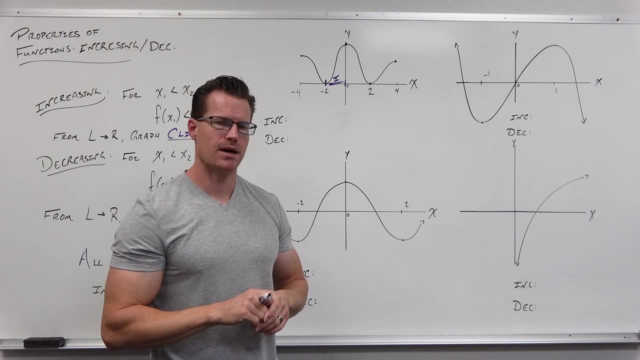 That's an interval of increasing. Then at 0,, it's well at 0.. At 0,, am I increasing? at that point, Am I decreasing at that point? Well, no, This is the reason why our intervals have to be. 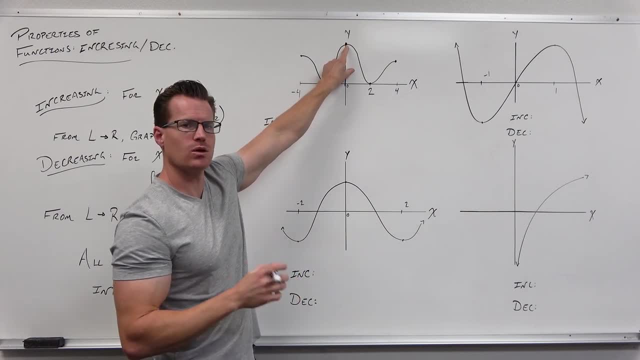 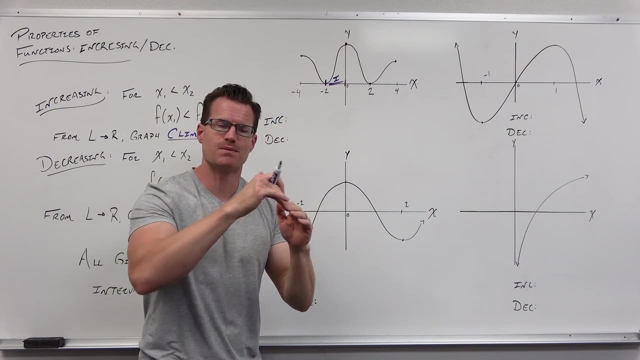 open At 0,. I'm neither increasing nor am I decreasing. That's called a local max. We'll talk about it next time, in the next video, But this is where we will change from increasing to decreasing. So we have this idea of open intervals for increase and decrease, because you 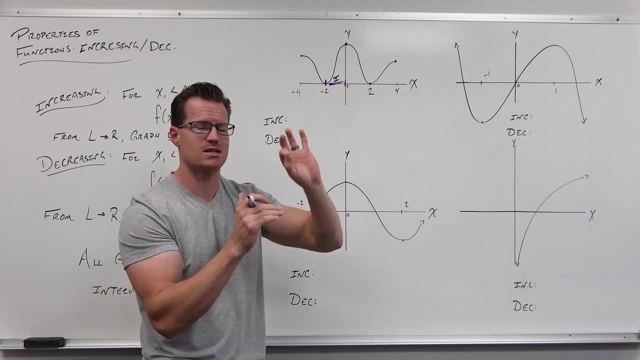 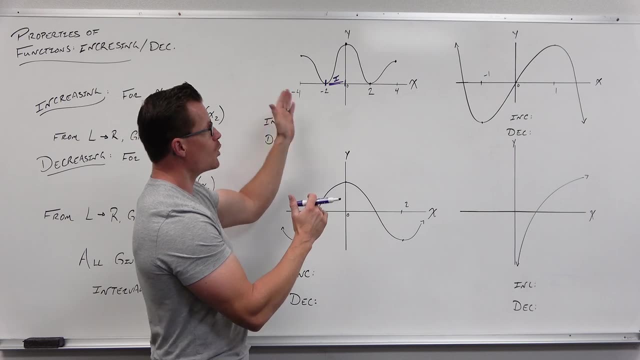 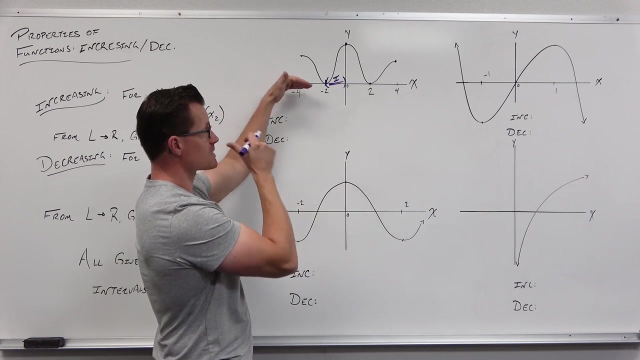 have the ability to get larger with every point that you're checking. Every x value that gets larger, your function must get larger for increasing, must get smaller for decreasing. So we have this open interval from negative 2 to 0 where our graph was climbing as I'm looking on. 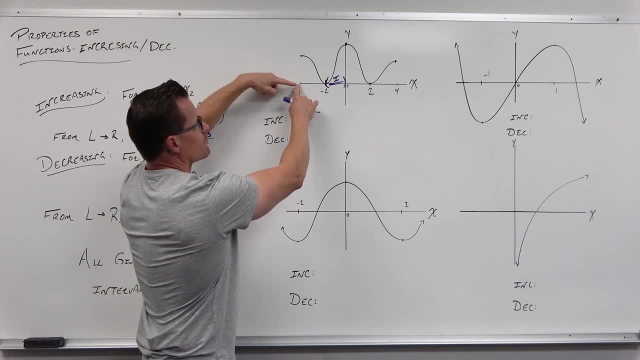 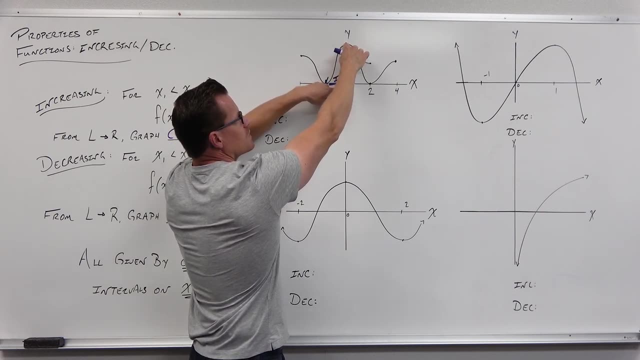 the x-axis. from left to right There's another one. So here I'm looking from here to here, My graph is falling, Then from here to here we're increasing. No problem, It's climbing From 0 to 2,. 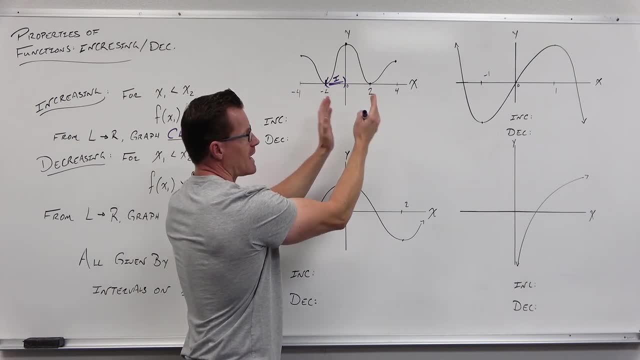 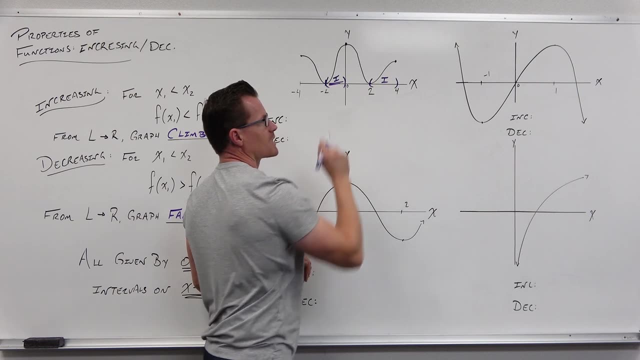 I'm falling. And then the next section of the graph where I look at my x-axis and my graph is climbing as I move from left to right, is from 2 to 4.. This is another section of increasing. My graph is climbing on this portion of the x-axis as I move from left to right. So when I put all 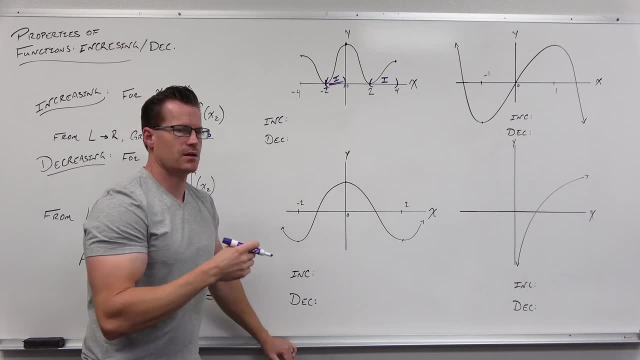 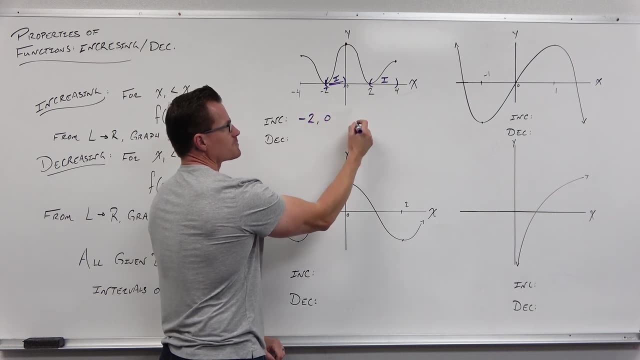 this together and we say that the intervals of increasing are the parts of the x-axis where, when I look from left to right, my graph is climbing. That's from negative 2 to 0.. That's also from 2 to 4.. 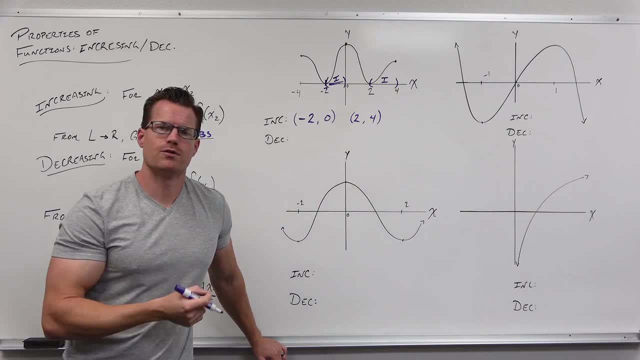 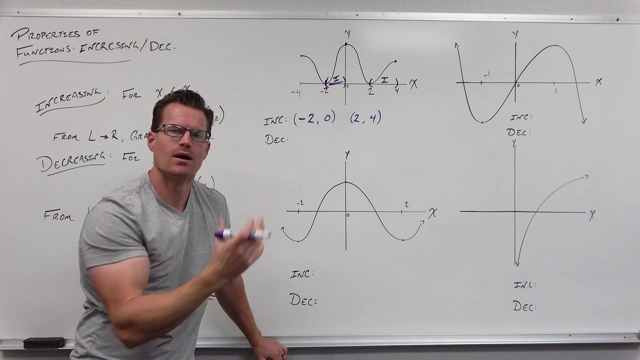 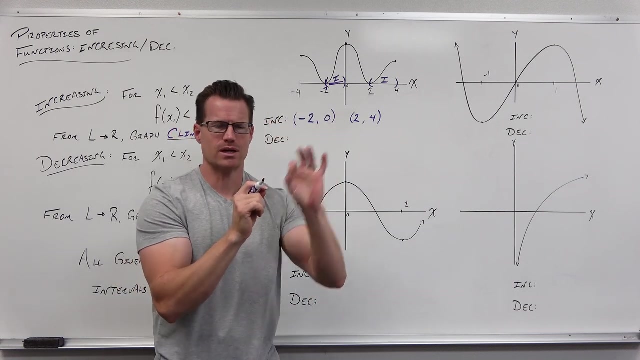 So we must use open intervals for all of those sections of the x-axis. It's a climbing idea. It doesn't have climbed and then you stop here. You always have to have an open interval so that you can satisfy this, so that there's a next point, and there's a next point, and there's a next point. 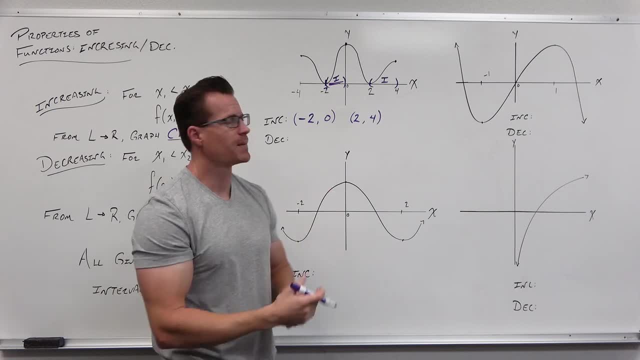 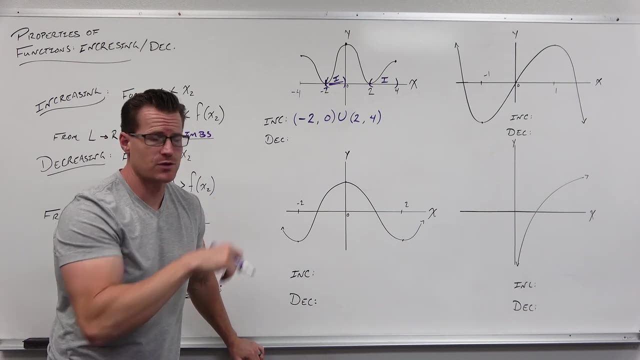 Open intervals. let you do that, Get as close as you want without actually stopping, And so to do that, we've got to have open. Decreasing is the opposite idea. So as you're still moving from left to right, But as you're moving left to right, your graph is falling. So find the intervals on the x-axis. 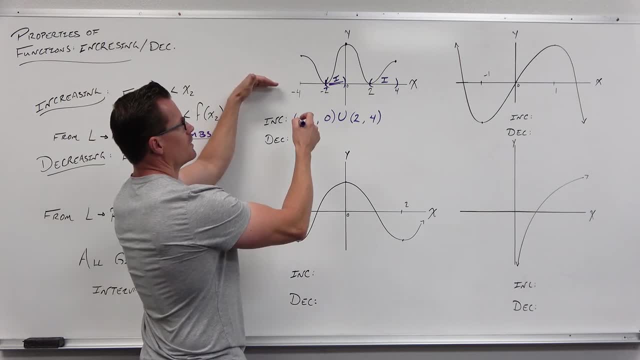 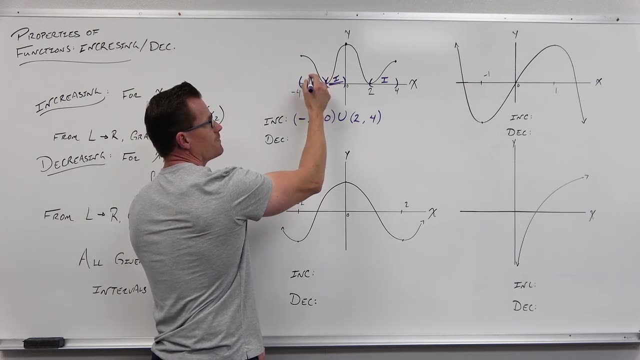 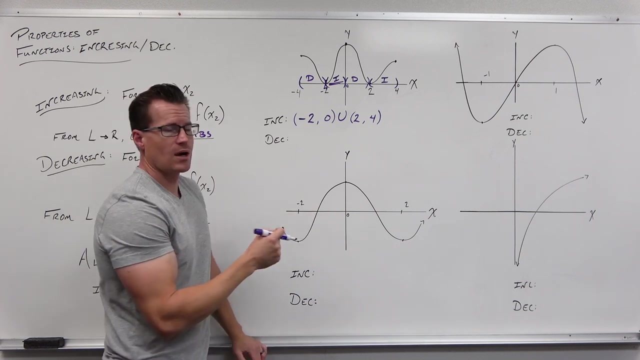 where, when I look from left to right, my graph is falling. Well, my graph starts at negative 4 and it's falling until we hit negative 2.. So this right here would be an interval of decreasing and another interval of decreasing, So our graph decreases. In this case, our graph is decreasing. 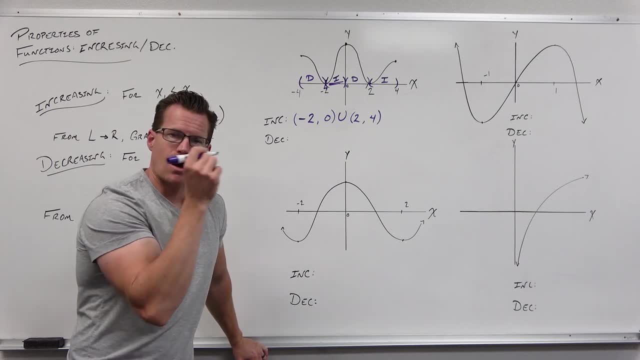 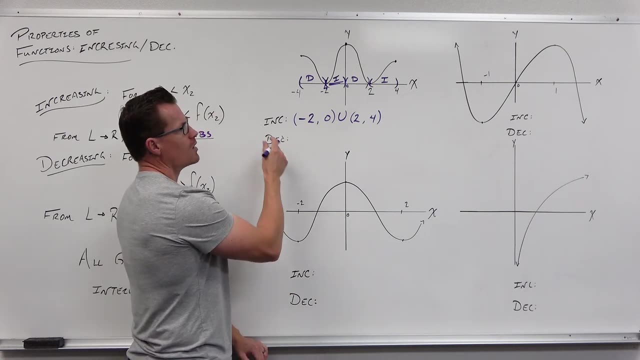 wherever it's not increasing. Sometimes you can have a constant, So where it's horizontal for a time, And then it will neither increase nor decrease, It'll just stay constant. We can deal with that too. But in our case here we have an interval of decrease in section x-axis where we're 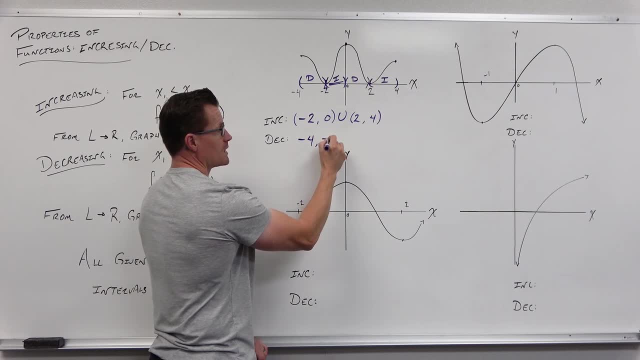 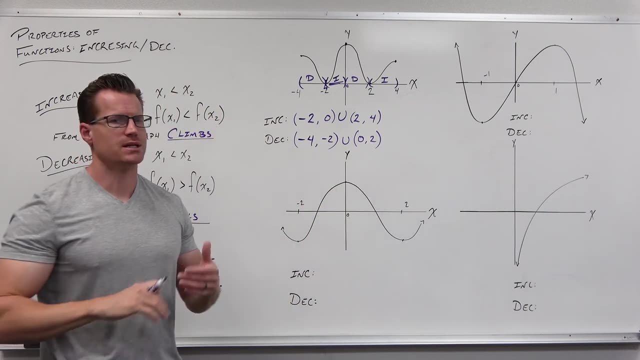 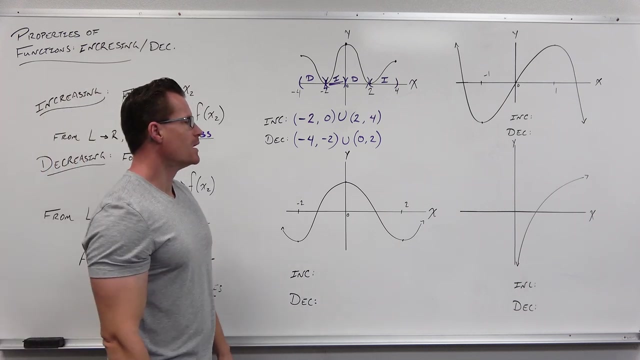 graph is falling as a read from left to right is negative 4 to negative 2. Open interval, Then again from zero to 2. That is how increasing and decreasing work. They're always open. They're always intervals of the x-axis, Super important for us to understand that. 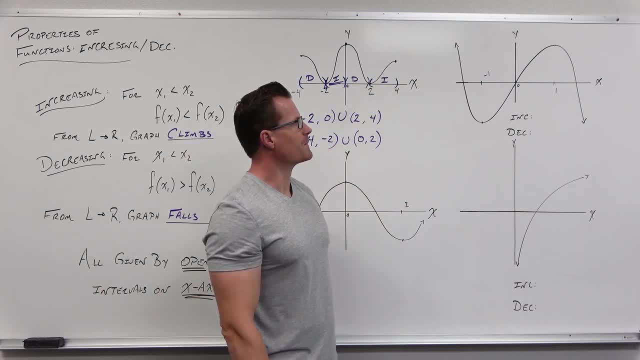 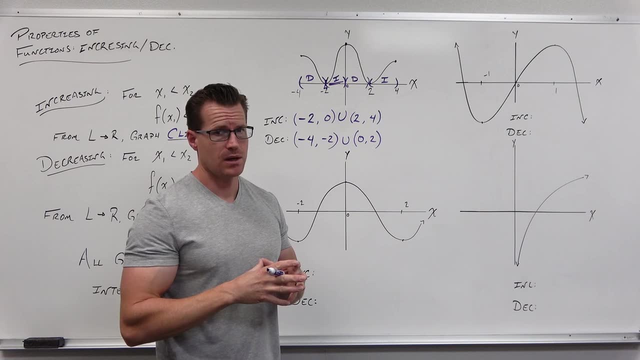 Let's go ahead and let's talk about the next one. We'll do this one over here. you look and see, man, you should be doing this. See if you can find the one interval of increasing. So the only interval of increasing is. I look from left to right on the x-axis where my graph is. 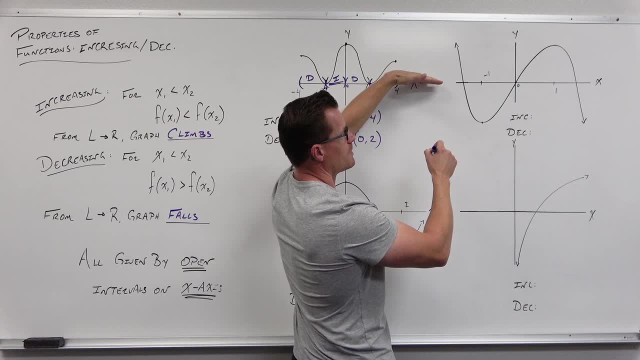 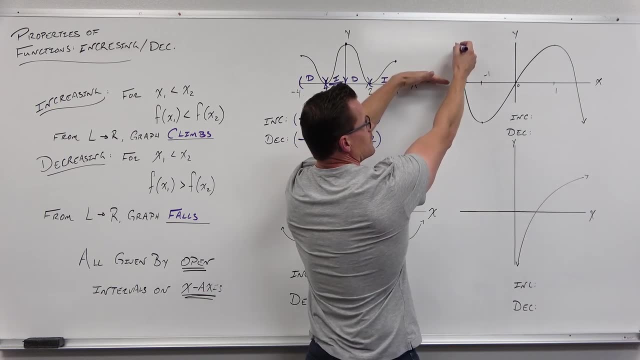 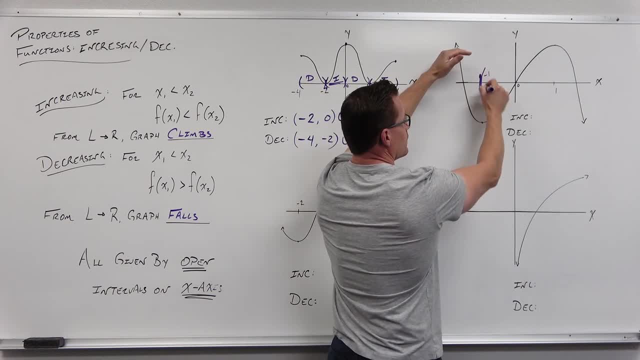 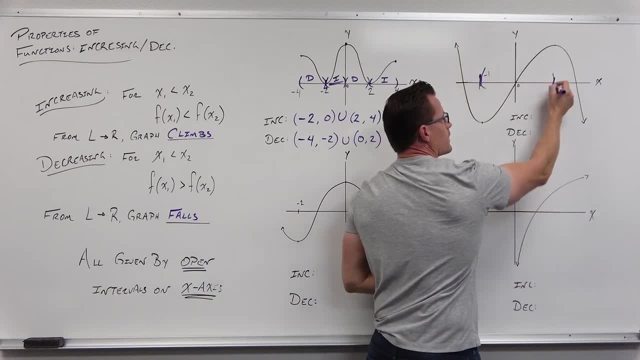 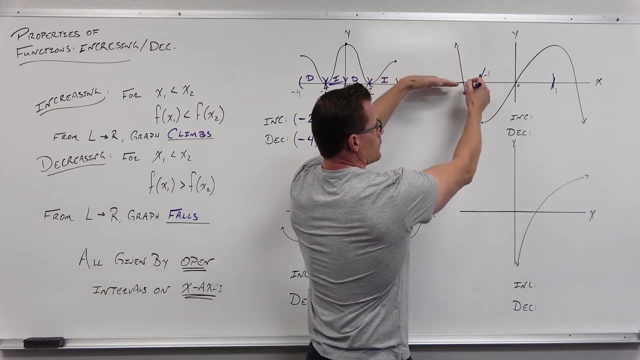 I'm going. Okay, I stopped increasing. Put another little mark. That right, there is how we determine the interval of the x-axis where our graph is climbing. So I was falling until I got here I started increasing. I stopped increasing. That right, there is my interval of increasing. It does. 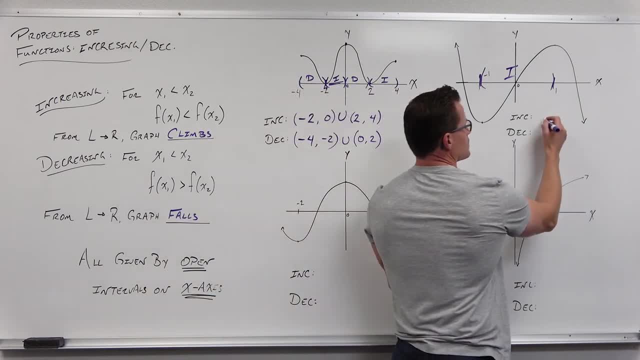 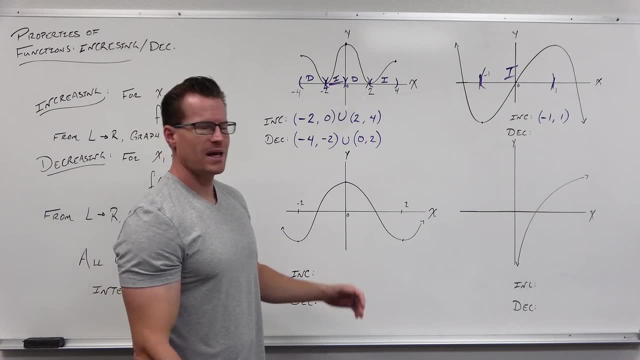 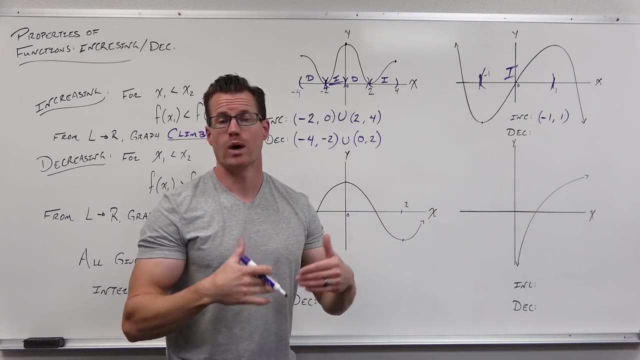 not increase outside of that. So interval of increasing is just from negative one to one, Now decreasing. it gets a little awkward when we think about what's going on here And the arrows they look confusing. Oh well, that's increasing. No, it's not. It's not increasing because the way 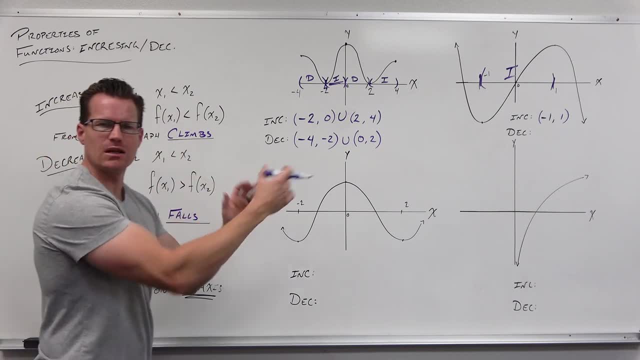 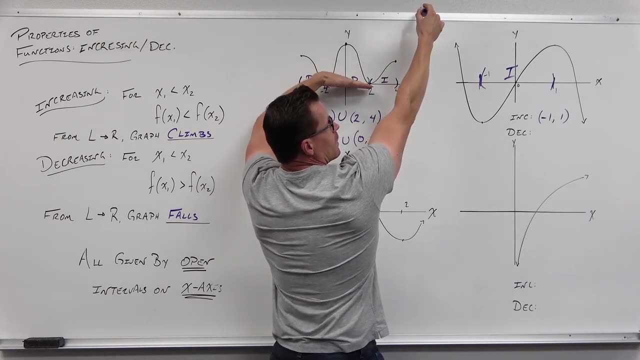 we read, our graph has to be from left to right as our x's are getting larger. So we put our hand on our x-axis and we go: okay, our graph is falling from where? Well, falling on the x-axis, this hand. 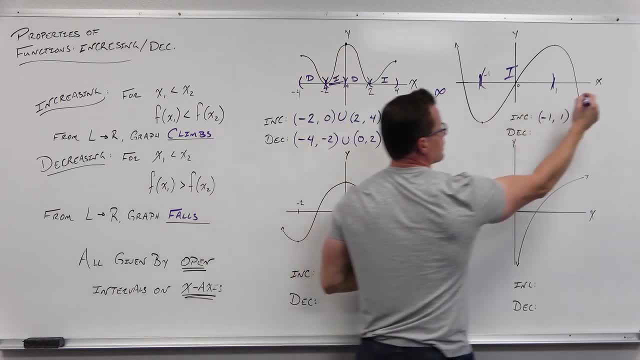 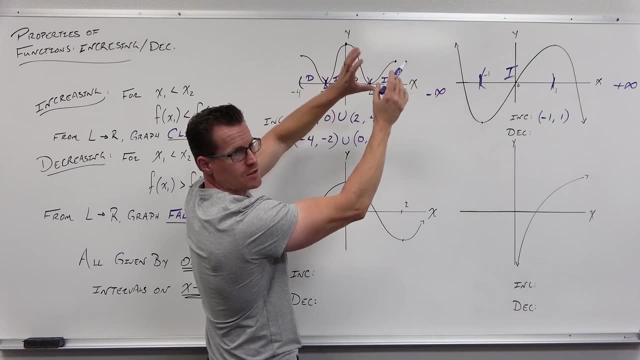 is way over at negative infinity. Negative infinity is over here and positive infinity is where Negative infinity is over here. Negative infinity is over here, Negative infinity is over here. So our graph is falling on the x-axis on that interval, The interval that this graph is. 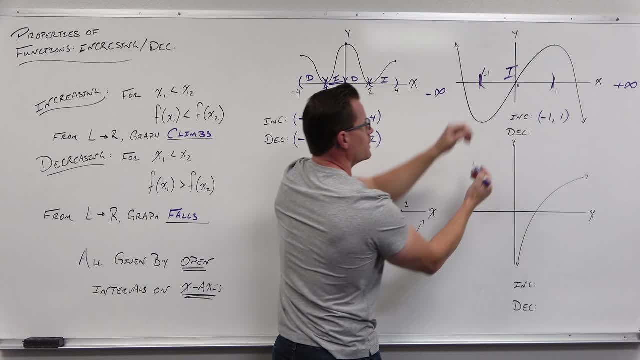 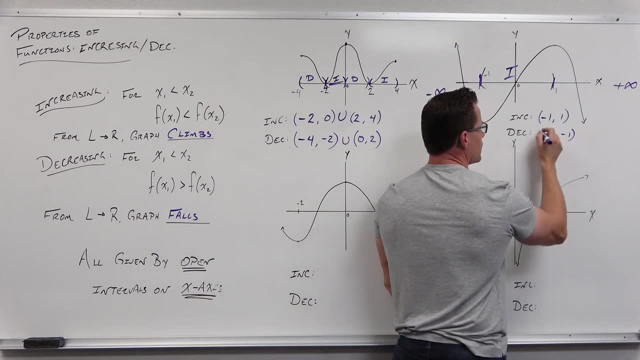 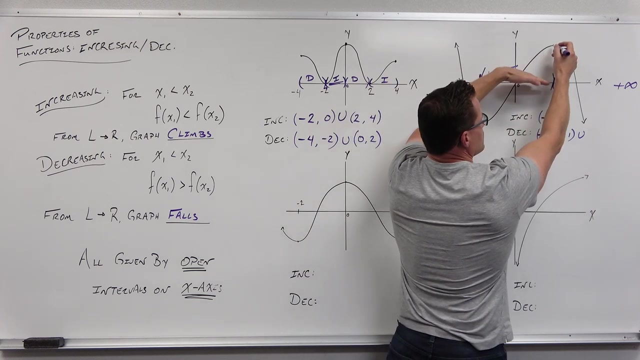 falling on is from negative infinity all the way until negative one. So, decreasing wise, this graph is decreasing on the x-axis from negative infinity to negative one, And then again. so let's see, Now I start to increase, I stop increasing. Oh, 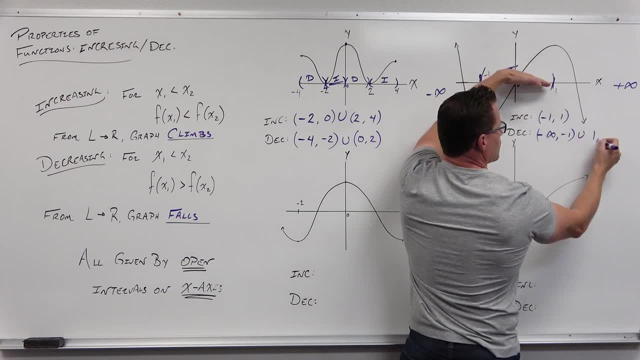 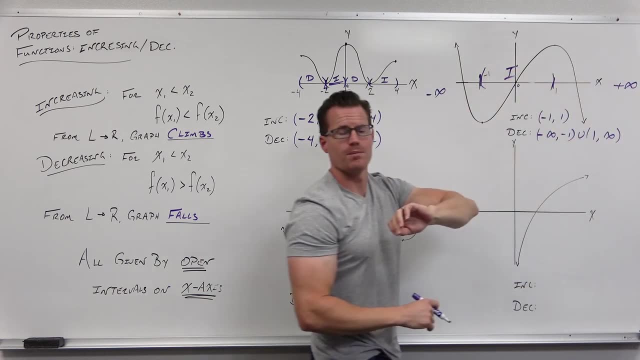 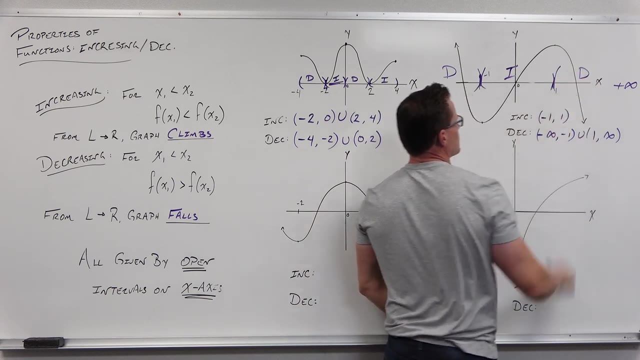 I'm starting to decrease again. So it's decreasing from one and then it never stops decreasing. It goes down, but my left hand keeps on with that x-axis forever. That's going to be decreasing into positive infinity. So we'd be decreasing here and decreasing here and it doesn't. 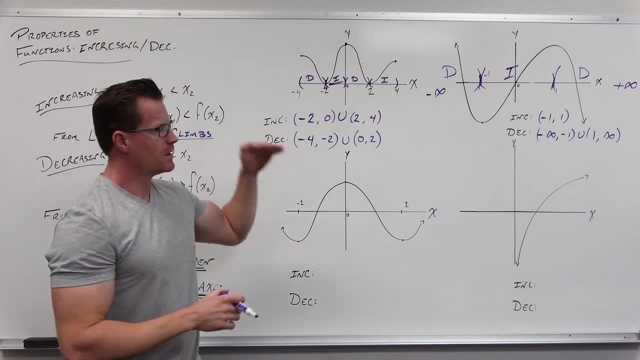 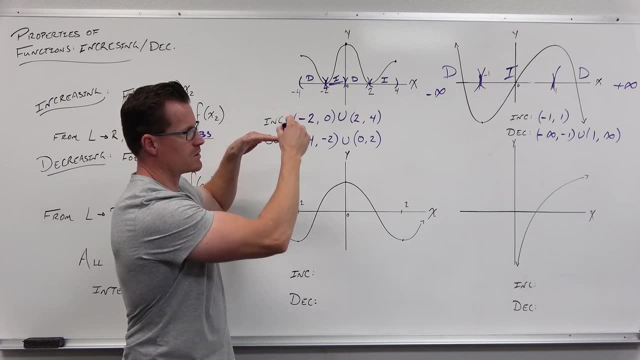 end. I hope that's making sense to you. I hope the idea of your left hand is kind of your marker. So where you're decreasing you're marking a decrease And then when you change, when you start increasing, make a little mark. So I'm decreasing and I start increasing. That makes. 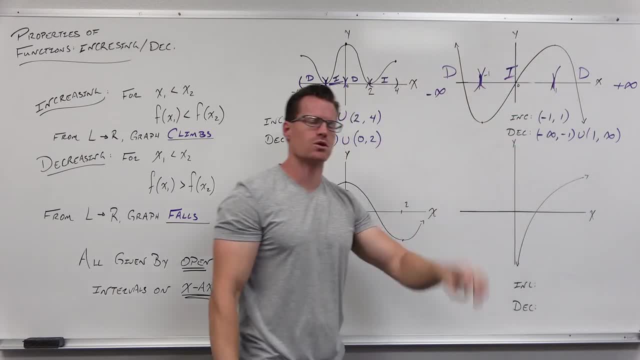 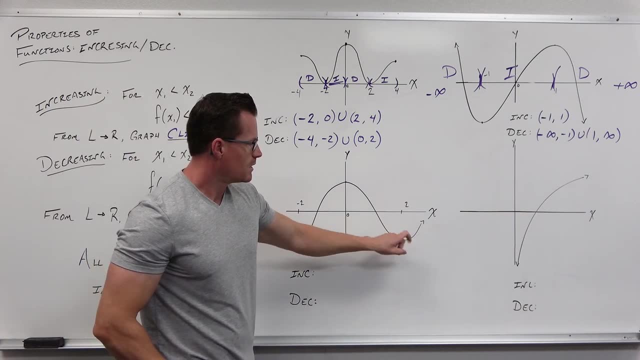 my little mark here Increasing, And then I stop And that's going to show you where your interval is. Okay, This one's, this one is tricky because of this right here, because it looks like sometimes we get some weird graphs and we have to kind of assume where it crosses the x-axis. 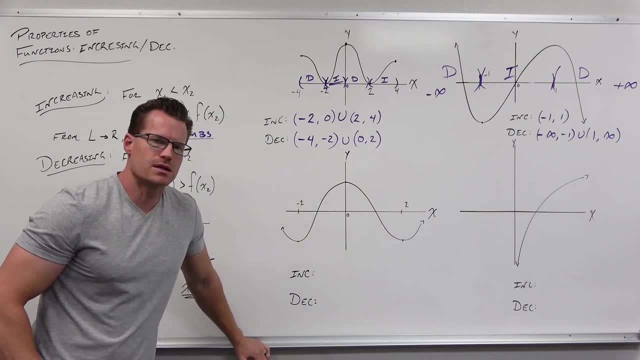 so that it keeps on going forever. You should be looking at this and finding your intervals of increasing. right now, You should be looking at that, finding increasing. So, as far as finding increasing, I'm going to trace the graph with my my right hand. I'm going to look at my left hand. 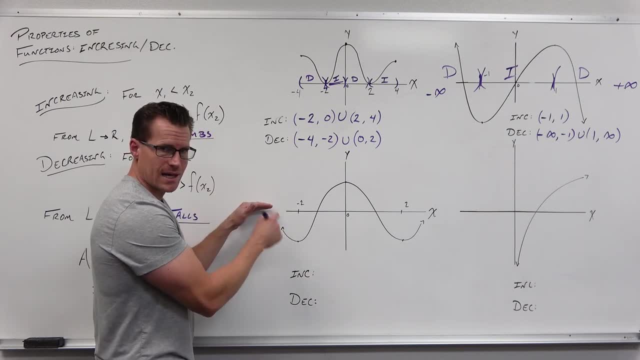 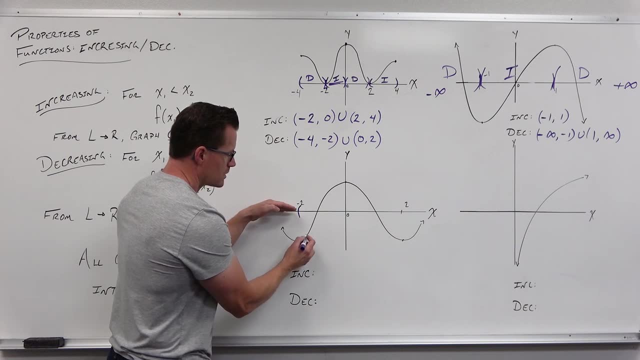 as it starts to climb As I move from left to right. that starts my interval on the x-axis for increasing. So I'm falling. here I'm falling right here I start to increase. So I'm going to increase, increase, increase, increase, I'm falling. This is my left hand. I'm hitting this. 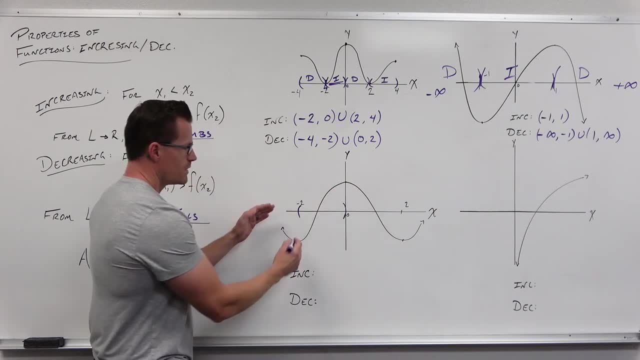 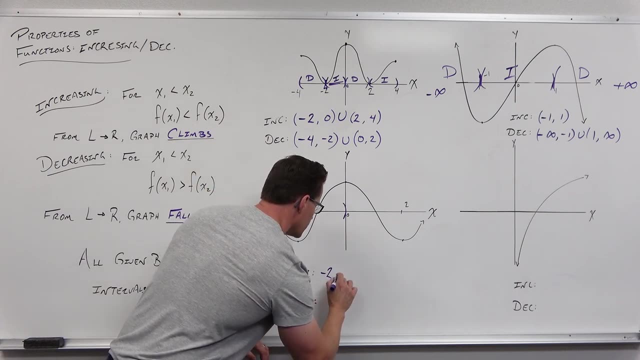 going: oh, now I'm going to start to decrease, I'm going to stop that. So this first interval from negative two to zero, that part of the x-axis is where my graph is climbing. So again, I'm at zero now. 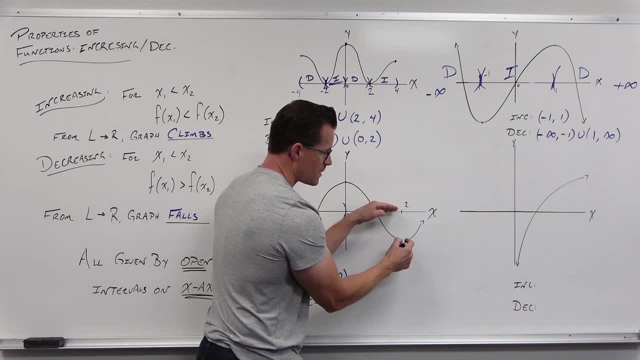 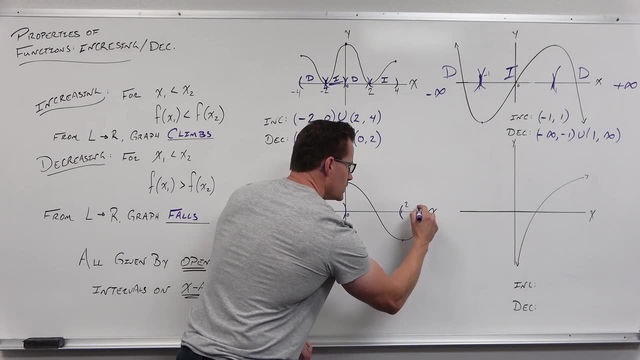 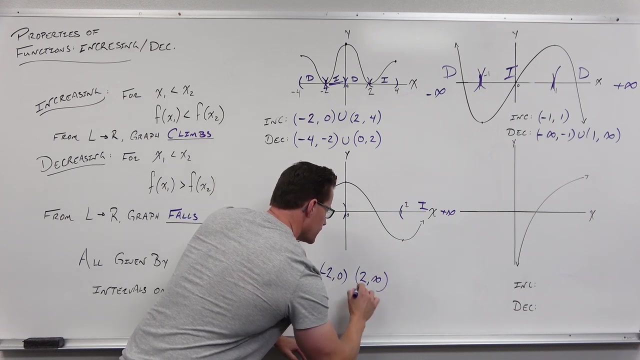 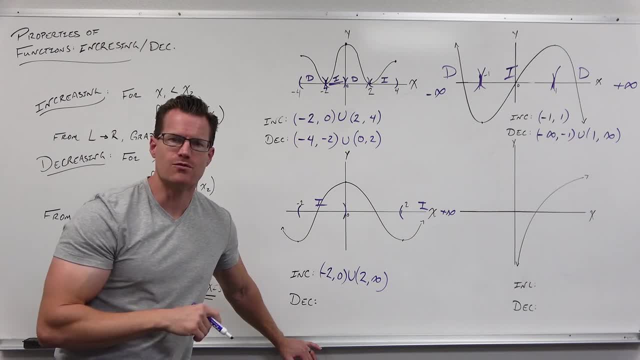 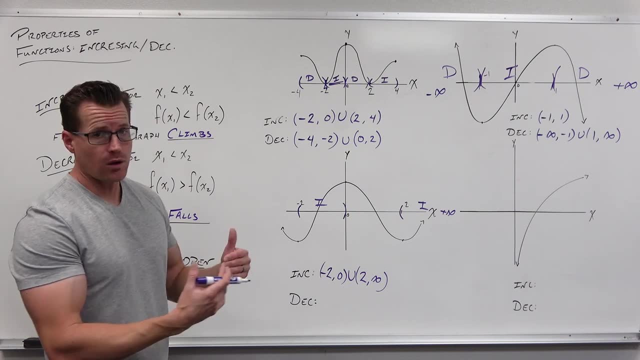 climbing. That's exactly what we're showing. They're always open. They never include the values because of the definition that we have for increasing and decreasing. I'm going to show the intervals on x-axis where I'm falling. So again, I'm going to take this. 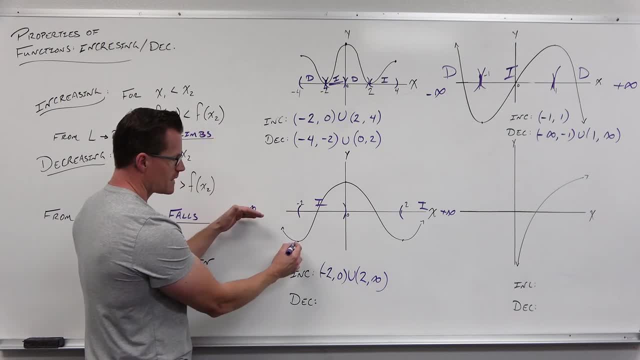 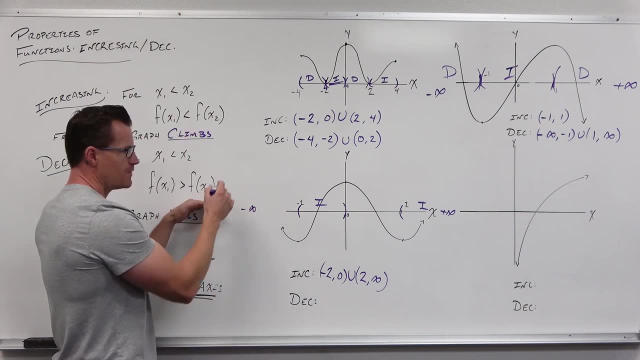 oh, yeah, hey, I start off falling. And because this goes forever, it will eventually get. remember, x-axis idea is one dimensional, It'll eventually get to negative infinity. So this graph is way over here. It's falling, falling, falling, falling, falling, all the way to negative. 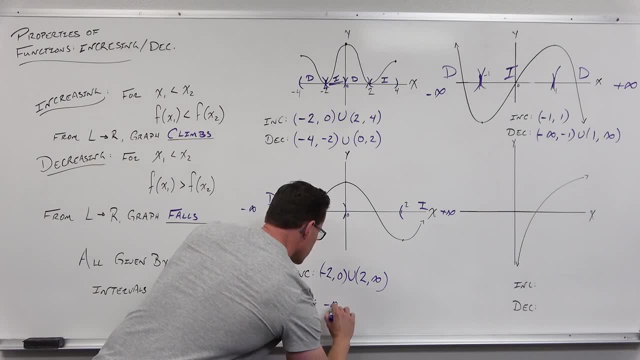 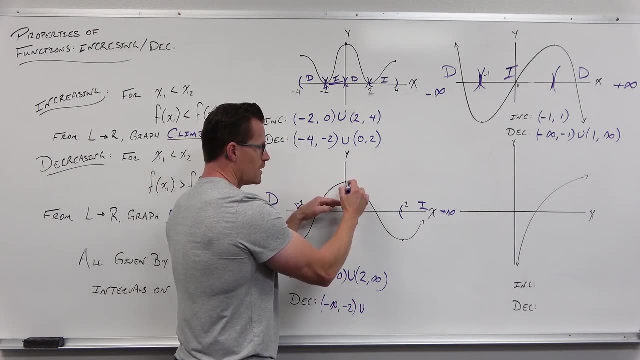 two, That's an interval of decreasing, And then okay. so now I'm increasing, increasing, increasing, increasing. Oh, it's starting to fall again, So I'm going to make another interval of decreasing until we get down to this point. 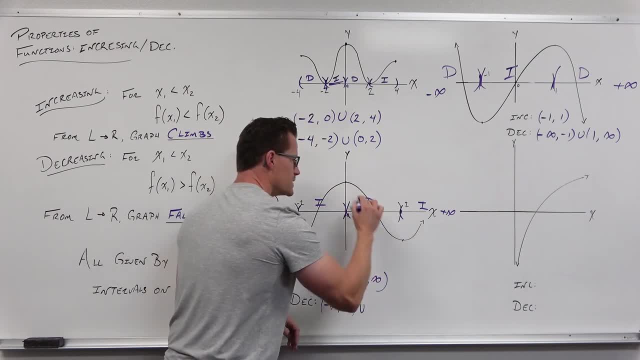 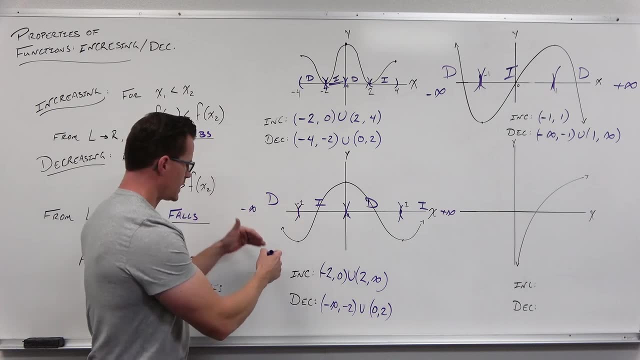 and on the x-axis until we stop at positive 2.. That's another decreasing from 0 to 2.. Are you seeing how to work that? Hopefully you're seeing how to make your interval. Your graph is doing one thing, but the intervals of increase and decreasing are only on the x-axis. 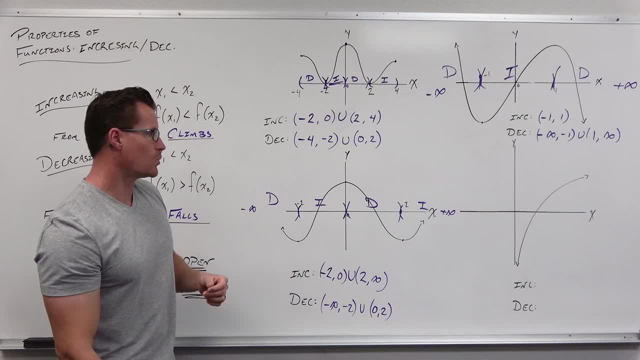 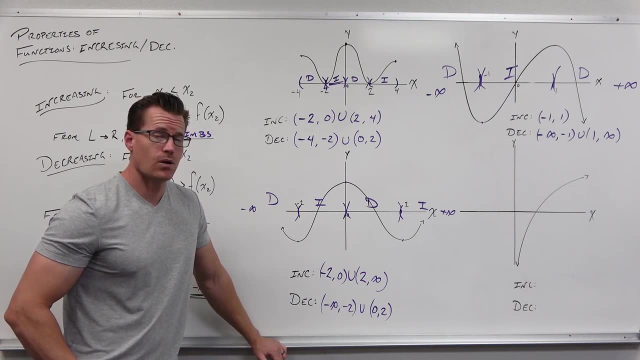 So only look one dimension when you're writing those intervals. Last one: is that graph ever decreasing? Is it ever decreasing? The answer is no, it's not, Because as we move from left to right, there's nothing going on here. 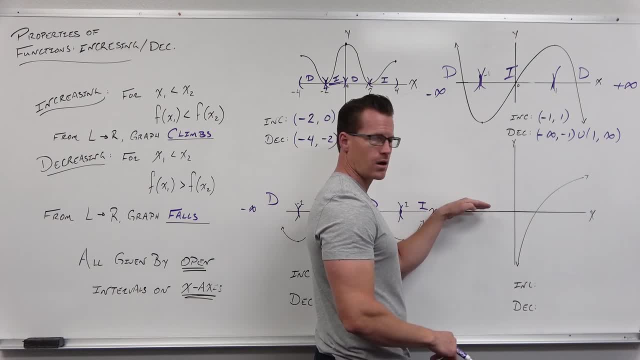 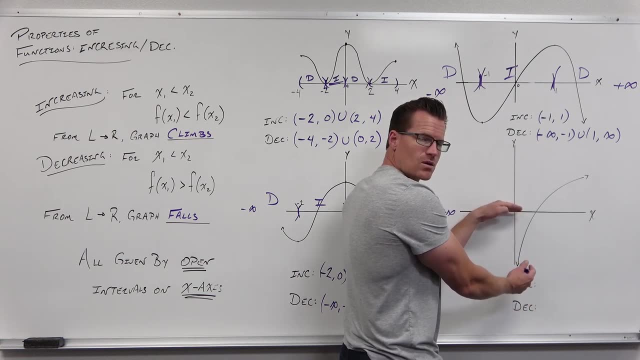 I want to include this interval at all, So I'm going. there's nothing going on. Why would I include that? There's no graph over here, But right when I hit that 0, oh, my pencil's down here. So at 0,. open interval here. 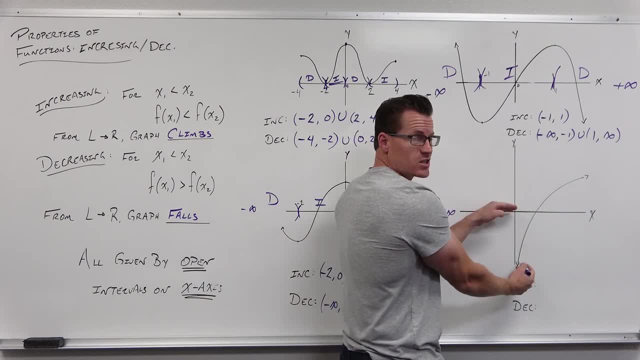 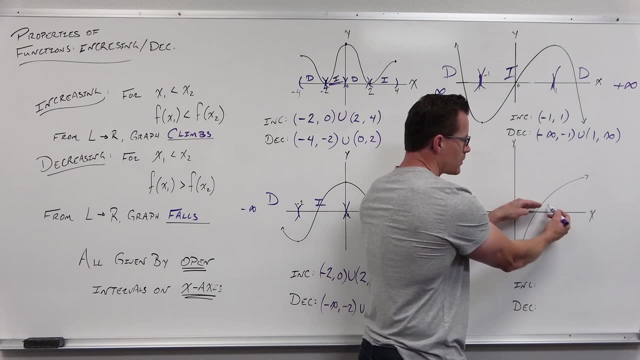 There's no point at 0. It's not defined, But just past 0, my pencil's way down here And as I trace this, my graph is climbing along this portion of the x-axis. It's increasing the whole entire time. 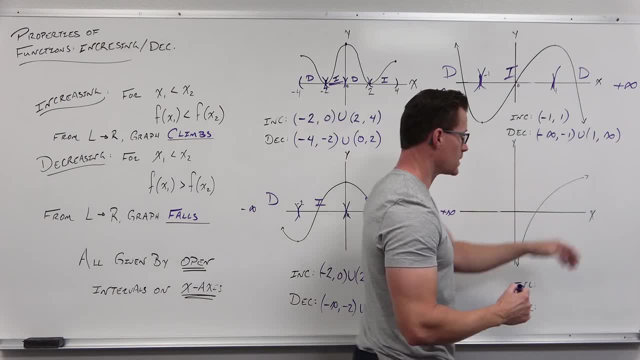 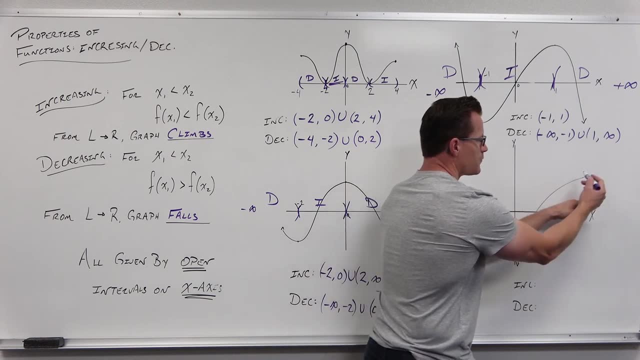 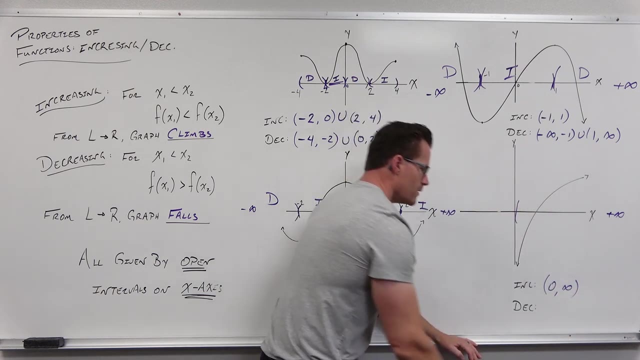 It'll never peak. It's going to get really slow, but it'll never peak. So this is increasing from. let's see again. It starts off at 0 and then it climbs forever. Open interval, there is no interval of decrease and it never falls. 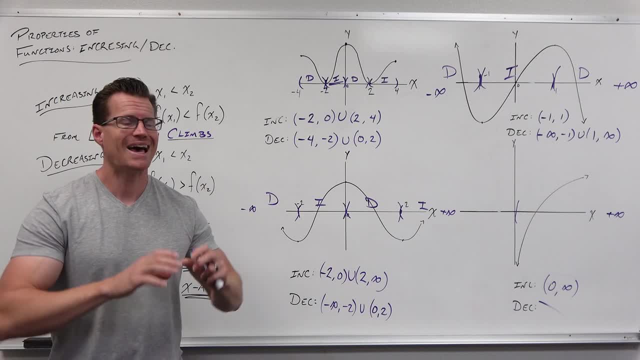 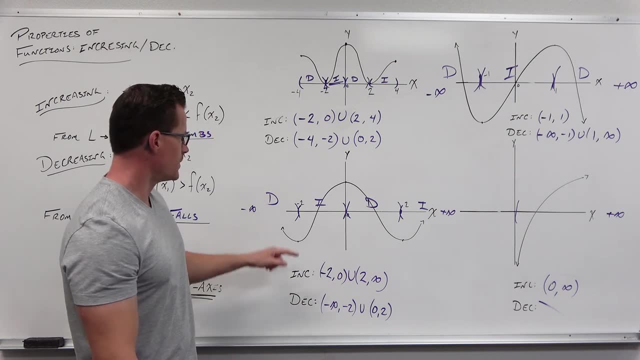 I hope that gives you a good interpretation of what increase and decrease mean, how it is always on the x-axis You can tell how easy it is for students to go. oh, it's increasing from negative, whatever this number is, to positive, whatever. 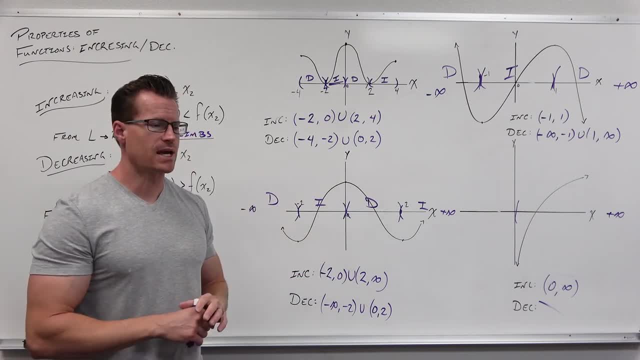 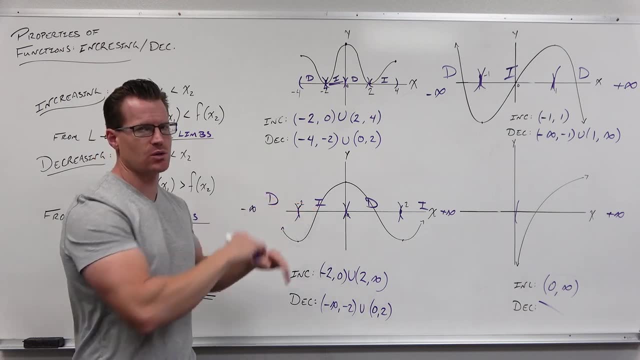 It's very easy to make that misconception. If we really focus on this as increase and decrease in our intervals of the x-axis, only where your graph is climbing do it the way that I showed you and typically that works pretty well. So that's going to be where we're going to stop on this video. 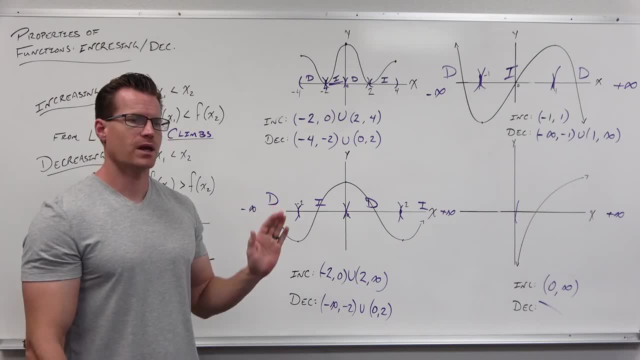 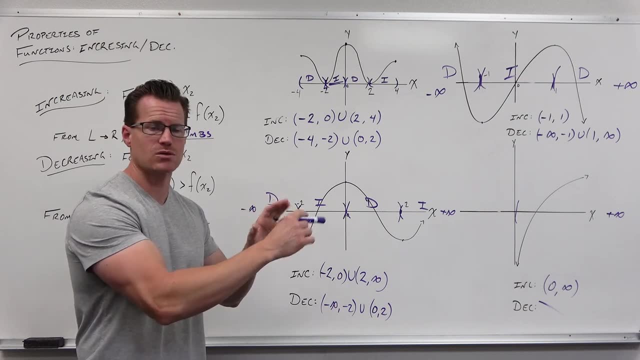 In the next video I'm going to talk about how, where we change from increasing to decreasing in a neighborhood around that point, we will have a peak, And in the neighborhood around where we change from decreasing to increasing, we'll have a little drop.